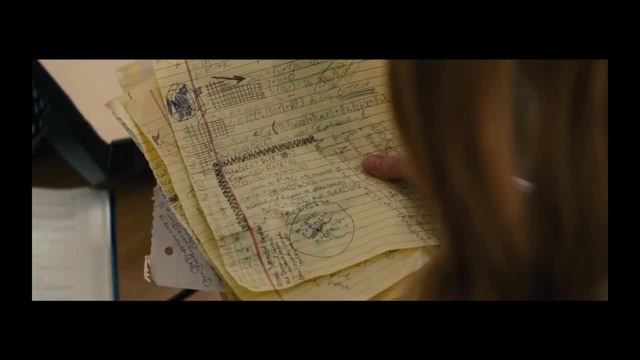 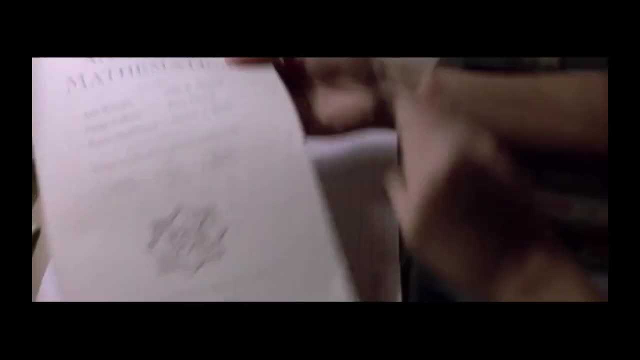 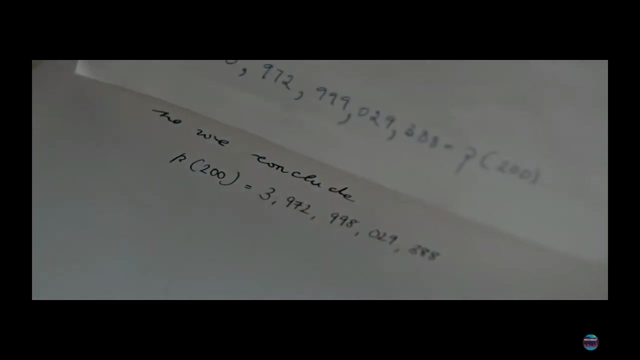 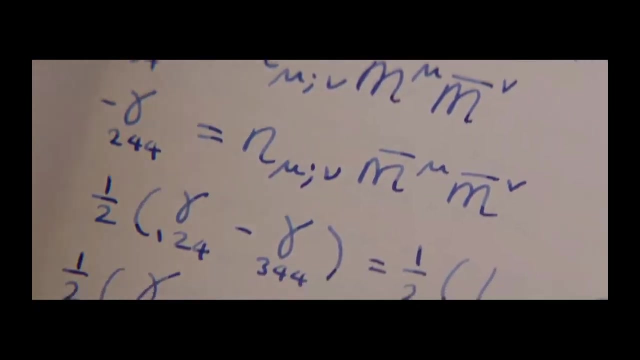 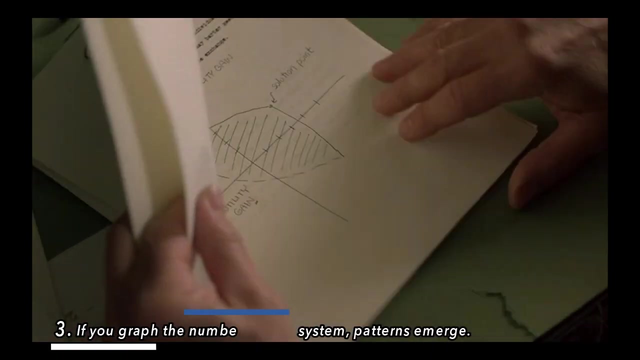 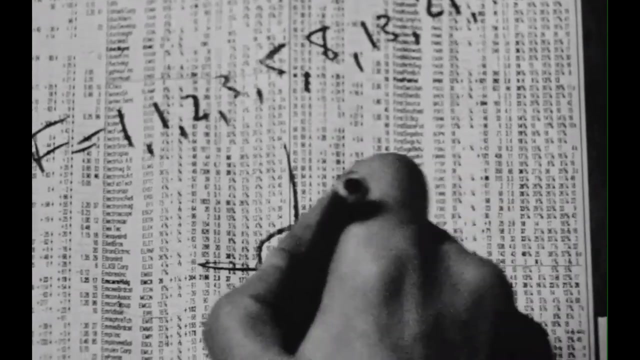 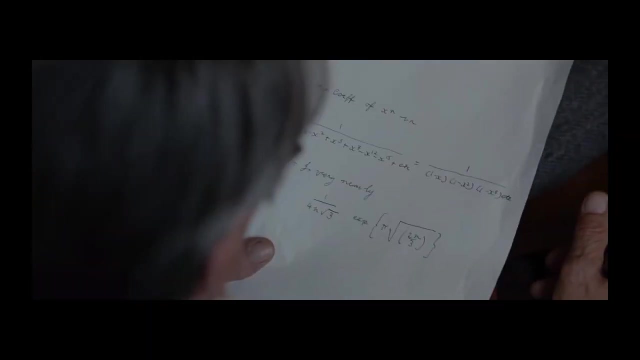 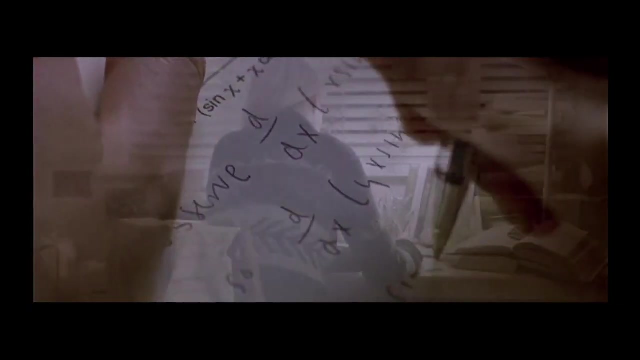 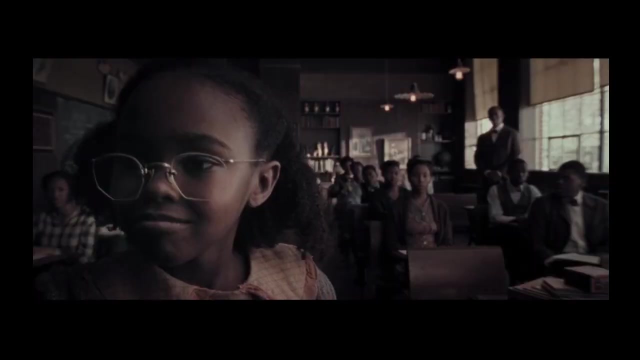 1. Mathematics is the language of nature. 2. Everything around us can be represented and understood through numbers. 3. If you graph the numbers of any system, patterns emerge. Therefore, there are patterns everywhere in nature. 4. If you're a human, feeling the presence of your sense of time. 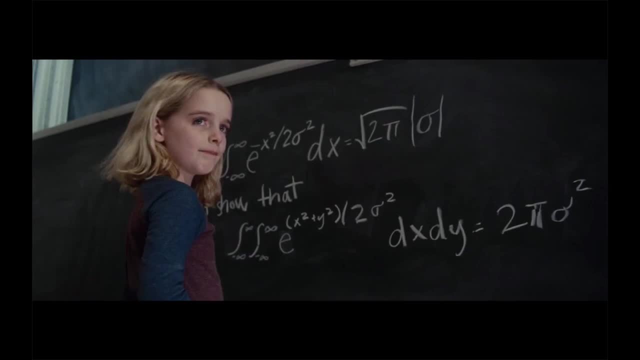 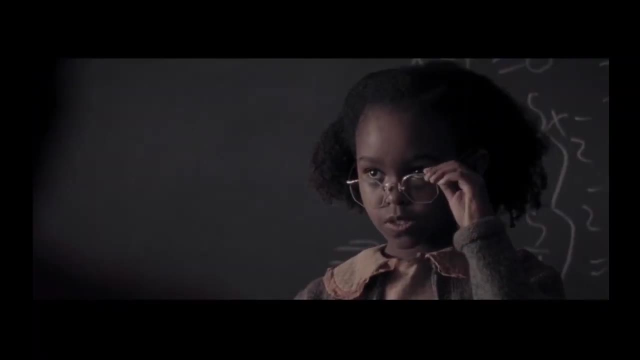 5. If you're a human, thinking about your sense of time. 6. If you're a human waking up from your baby, feeling comfortable. 7. If you're a human, lovingly feeling like you're better off- Scalene. 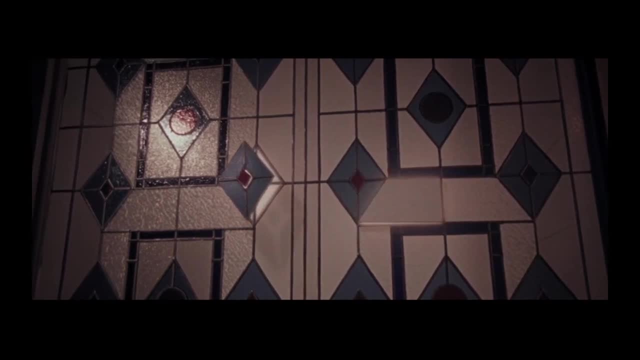 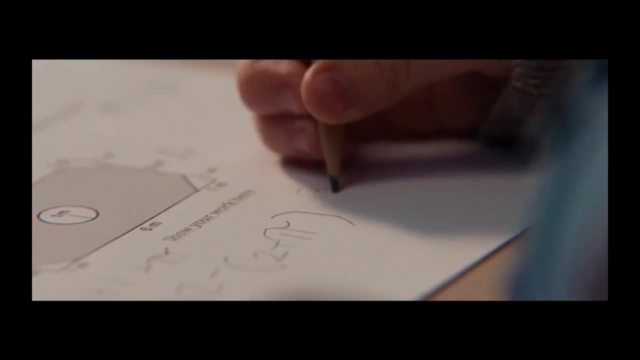 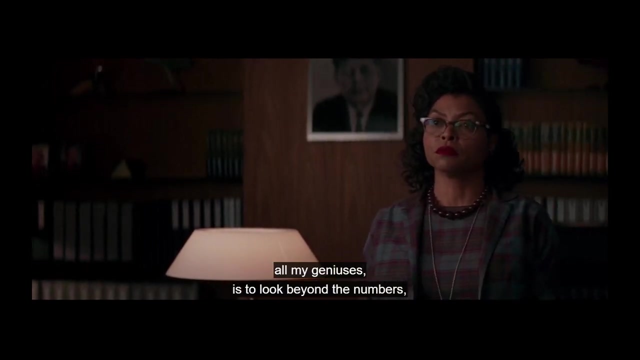 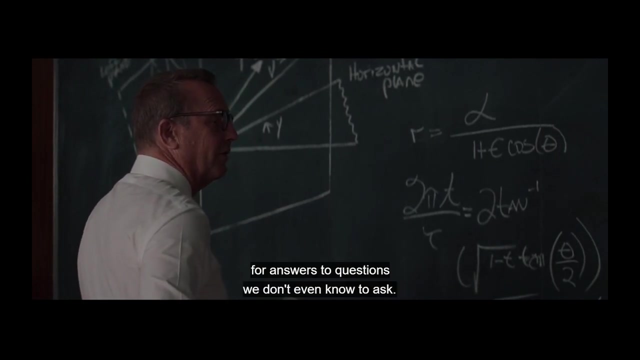 Echolateral Rhombus Trapezoid. What I'm asking you to do, what I'm asking everyone in that room, all my geniuses, is to look beyond the numbers, to look around them, through them and answer the questions. 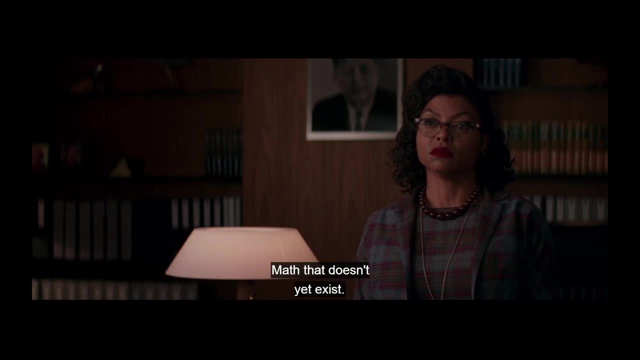 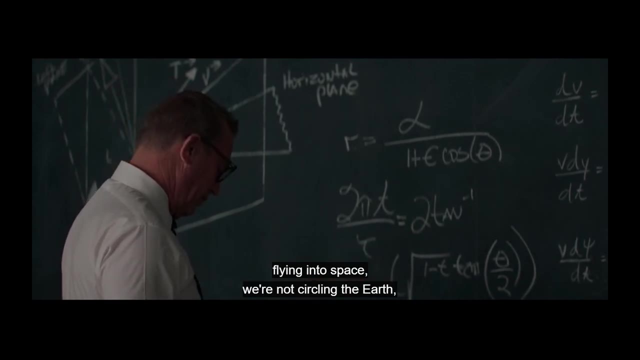 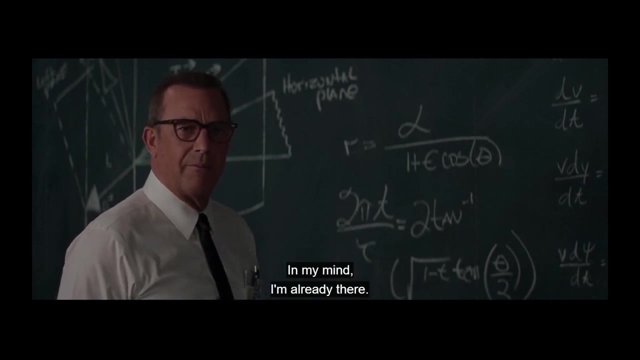 we don't even know how to ask math that doesn't yet exist, because without it we're not going anywhere. I mean, we're staying on the ground, we're not flying into space, we're not circling Earth and we're certainly not touching it, but in my mind, in my mind, I'm already there. 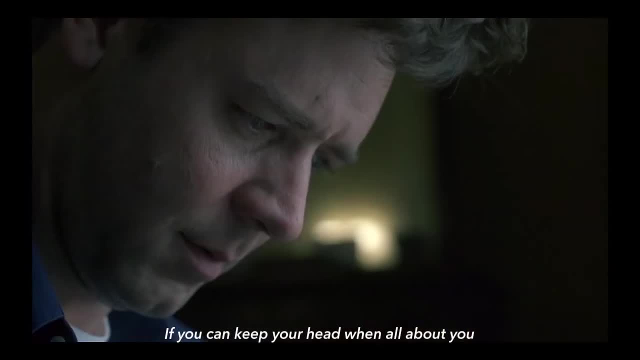 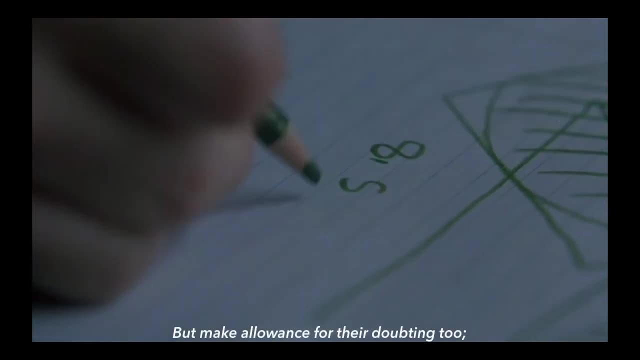 Are you. If you can keep your head when all about you are losing theirs and blaming it on you. if you can trust yourself when all men doubt you, then make allowance for their doubting too. If you can wait and not be tired by waiting. 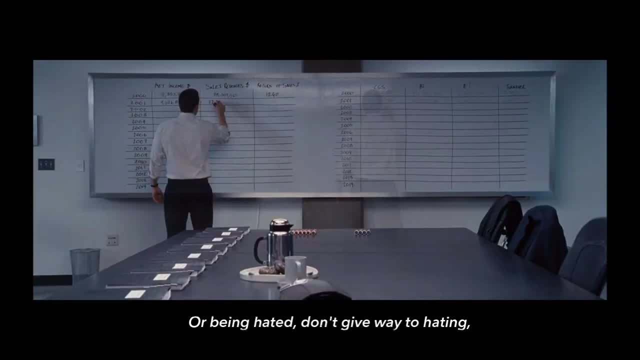 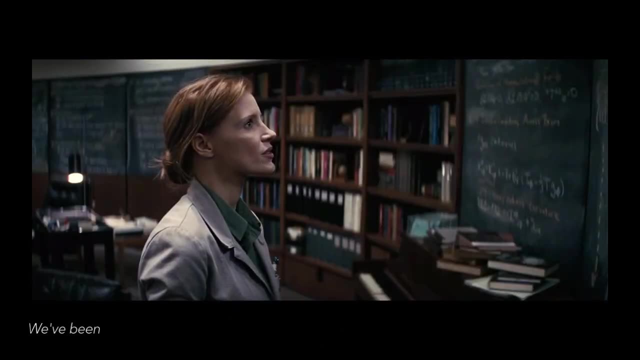 Or being lied about- don't deal in lies- Or being hated. don't give way to hating and yet don't look too good nor talk too wise. We've been trying to solve the equation without changing the underlying assumption about time. 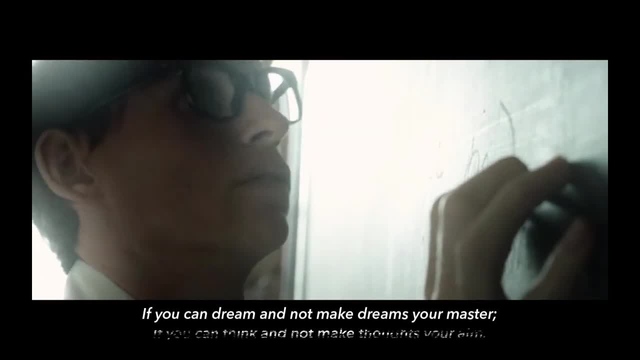 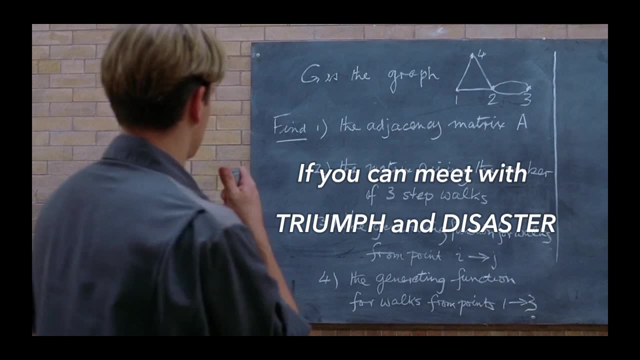 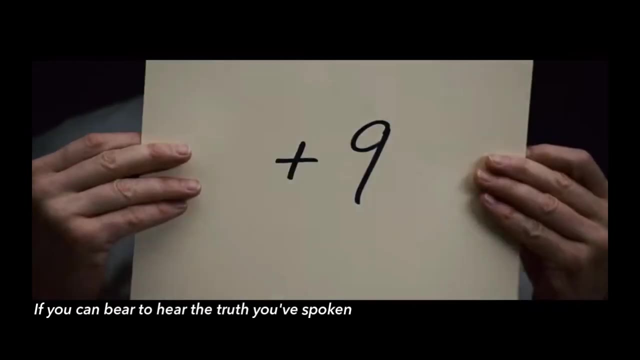 If you can dream and not make dreams your master. If you can think and not make thoughts your aim, If you can meet with triumph and disaster and treat those two imposters just the same, If you can bear To hear the truth. you've spoken twisted by knaves to make a trap for fools. 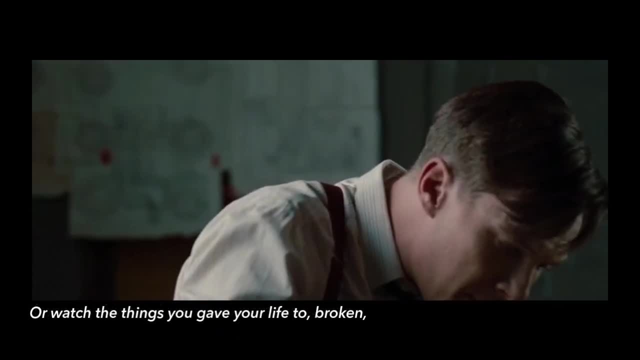 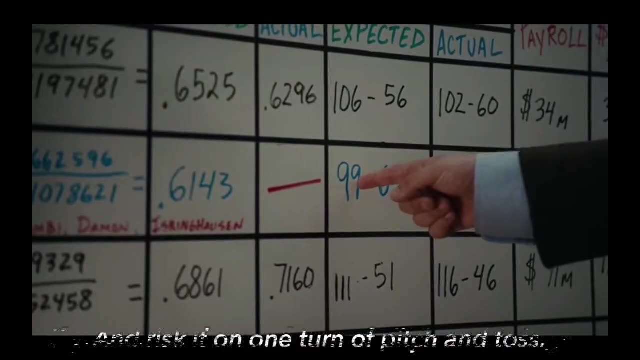 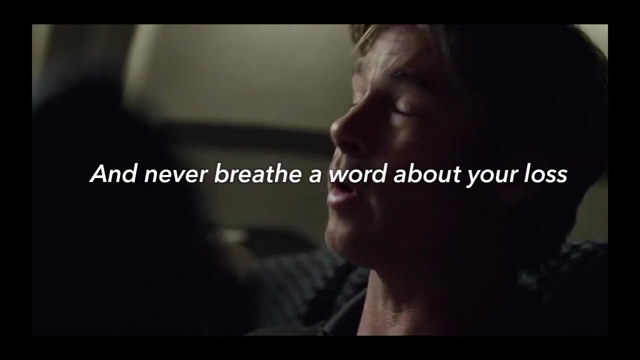 Or watch the things you gave your life to broken and stoop and build them up with worn out tools If you can make one heap of all your winnings and risk it on one turn at pitch and toss and lose and start again at your beginnings and never breathe a word about your loss. 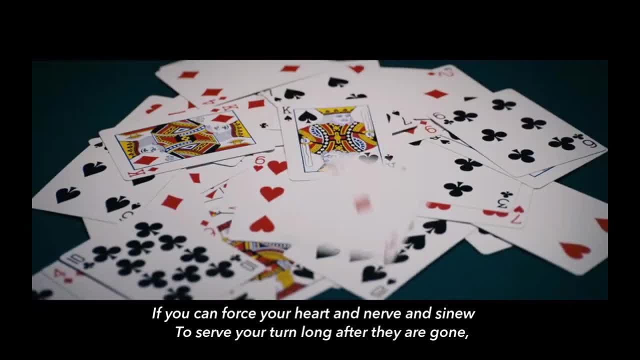 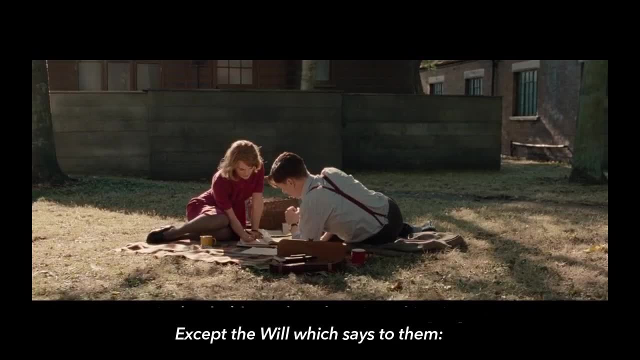 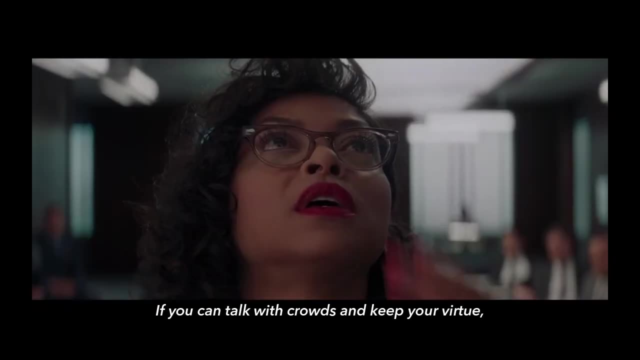 If you can force your heart and nerve and sinew to serve your turn long after they are gone. And so hold on when there is nothing in you except the will that says to them. hold on If you can talk with crowds and keep your virtue, or walk with kings, nor lose the common. 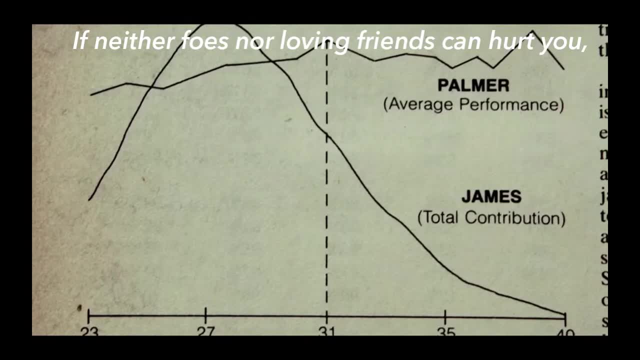 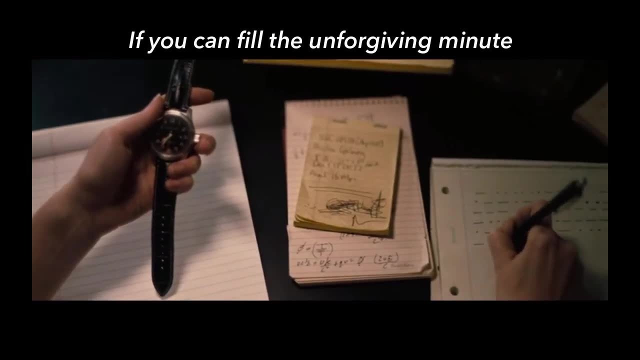 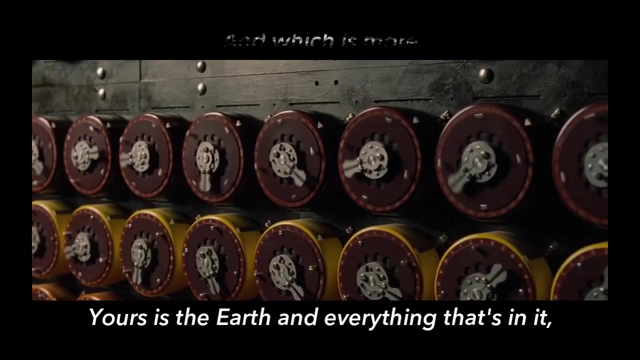 touch, If neither foes nor loving friends can hurt you, If all men count with you but none too much, If you can fill the unforgiving minute with sixty seconds worth of distance run, Yours is the earth and everything that's in it. 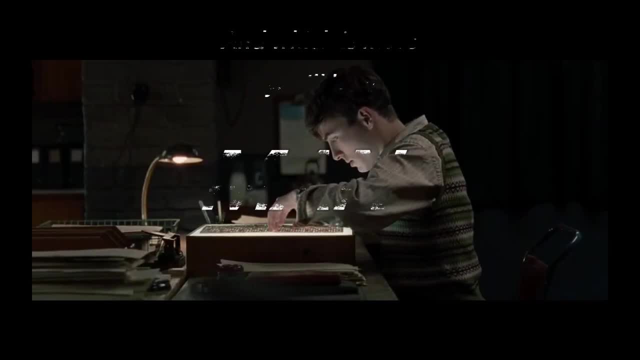 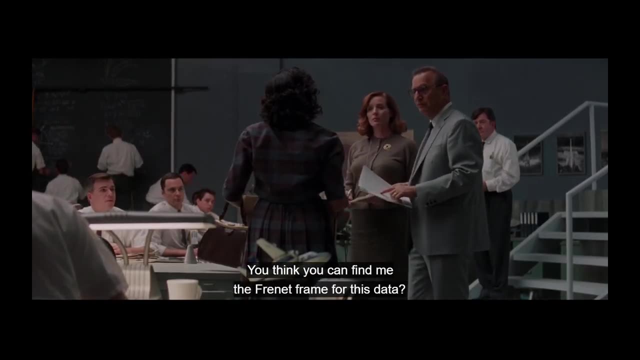 And, which is more, you'll be a man. my son Did you just solve, Riemann? You think you can find me. the Frenet frame for this data, The Gram-Schmidt- Orthogonization algorithm, Yes. 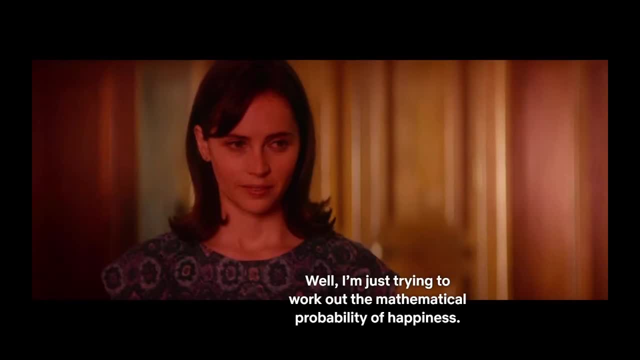 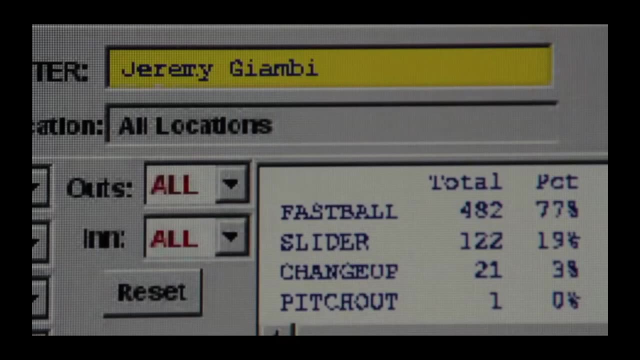 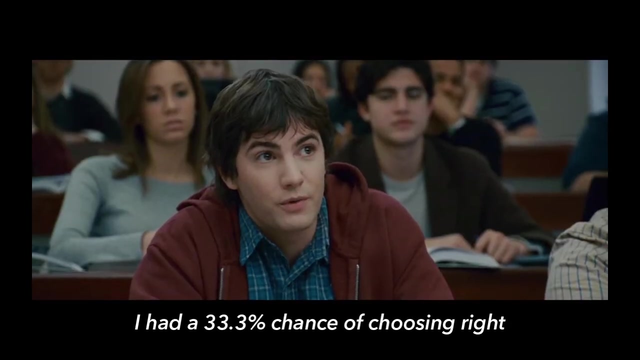 I prefer it over you calling in coordinates. Probability of happiness. You're close. Some integer is zero. but no, You were right. Cauchy's theorem will work. Before I had a 33.3% chance of choosing right.